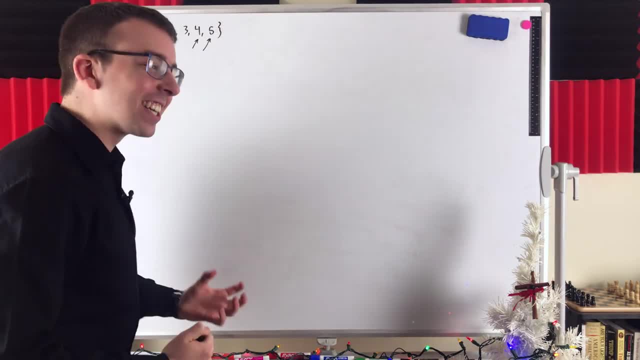 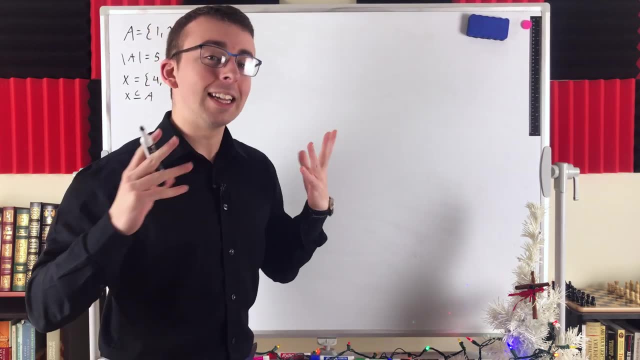 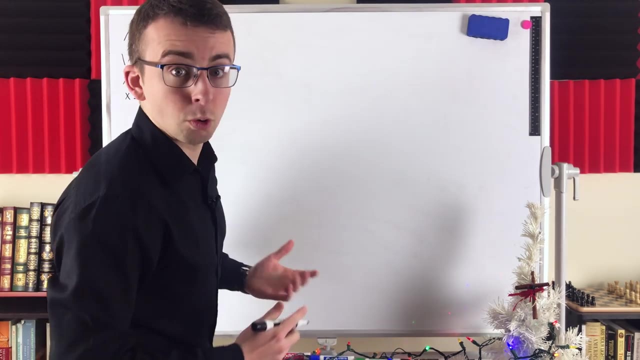 train is distracting, so loud just screeching at the top of its lungs. Let's roll right into something a little bit easier. Okay, 1 to 15.. Okay, So we begin with a more easy question, an easier question, which is: how many subsets of A? 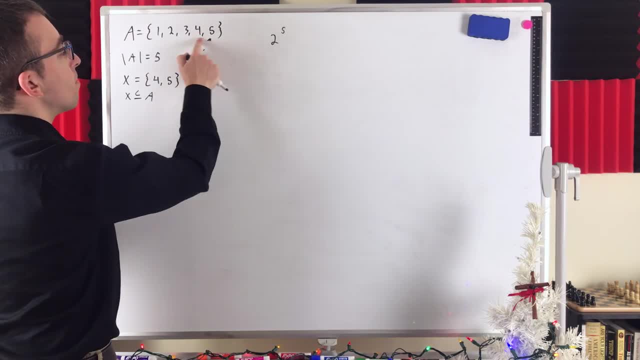 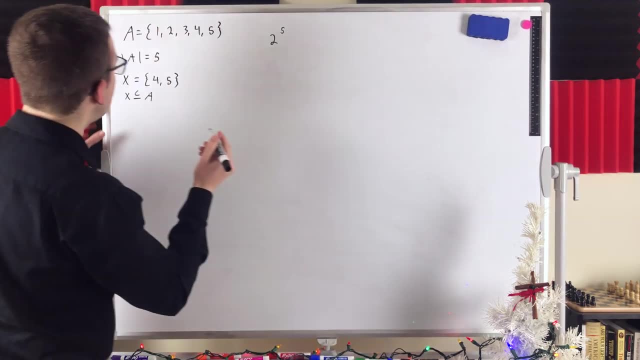 are there period Without any special rules. A lot of you already know. the answer is 2 to the power of 5.. It's 2 to the power of the number of elements of A. This is easily explained like this: When making a subset of A, we have two choices. for every element of A, We can include 1 in the group. and we will also put 1 in the pop up here and we will take the two assists and we're gonna have four options in the group and cdr something. Then, in particular, if the sub Lös a, they're got so many limit points between those 1's, how do they junct us to the next to 12th and 5th number We can give? 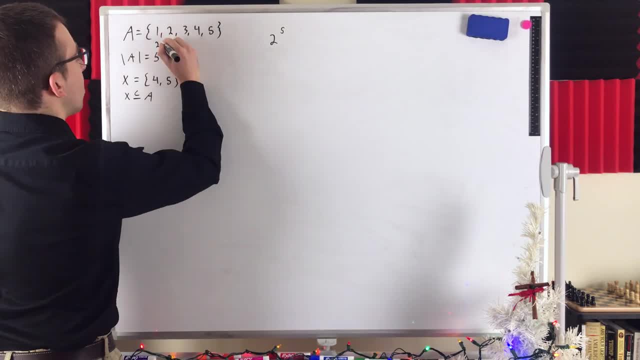 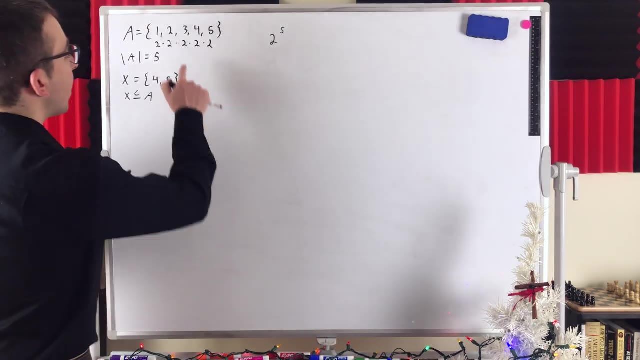 or we can not include one. For each of those two choices we have another two choices for the next element. We could include two or not include two, and so on. We have two choices for all five elements. The total number of subsets is two to the power of five. Then we can actually extend. 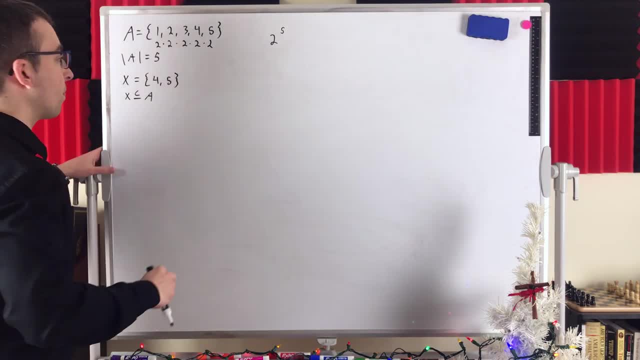 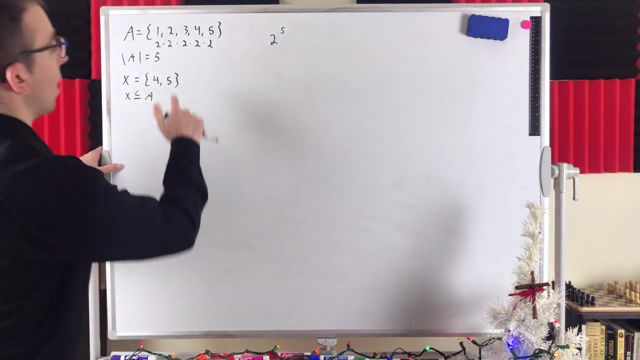 this logic to pretty easily answer our question. We have two choices. If we're trying to count the subsets, we're counting the subsets that include four and five. We have two choices for all of the elements except for four and five. We only have one choice for those elements because we're 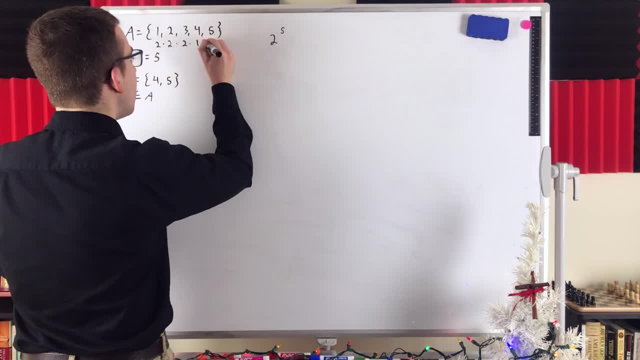 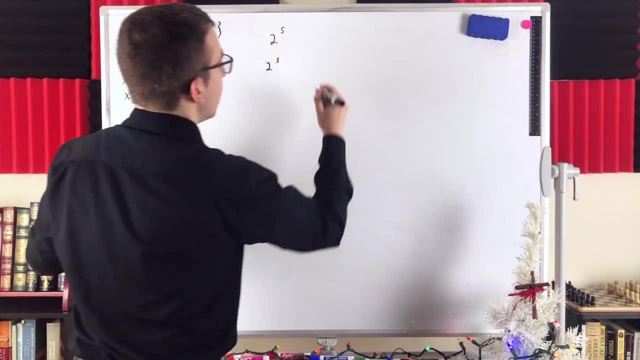 guaranteeing that we will include them, And so the answer becomes two times two times two times one times one, or two to the power of three. So this suggests the general solution. It's two to the power of the number of elements in the set. 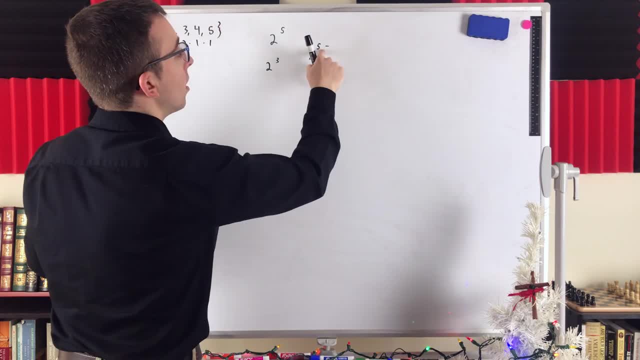 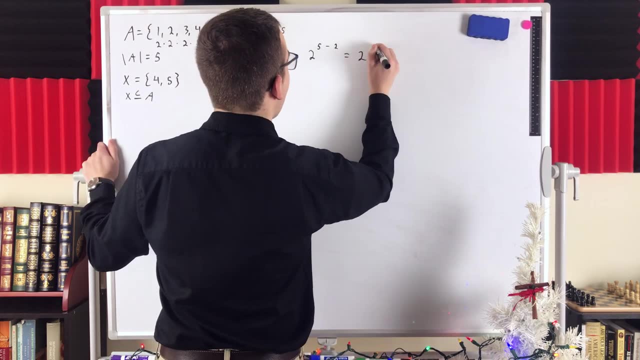 two to the power of five of 5 minus in the exponent, minus the number of elements we're guaranteeing we will include 5 minus 2, that's 2 to the power of 3.. You might also notice that the same logic would answer the. 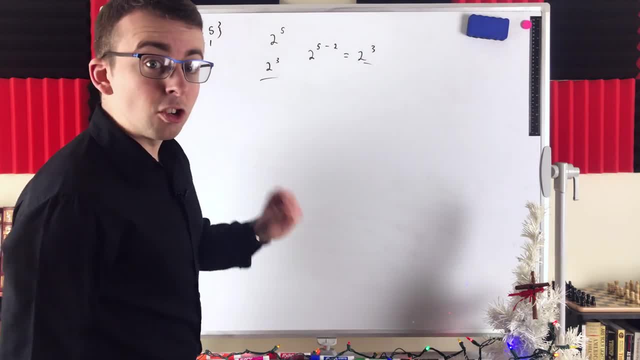 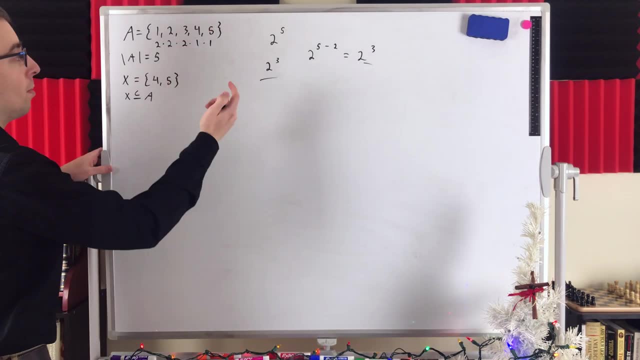 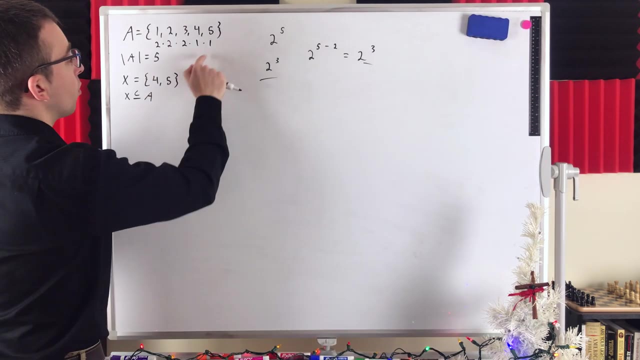 question: how many subsets of a are there that don't include 4 and don't include 5, so it includes neither of those elements? The answer would be the same, because we're saying we have two choices for one, two choices for two, two choices for three, but again we only have one choice for four. and 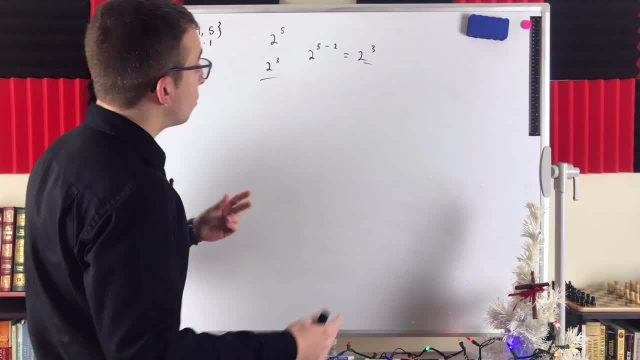 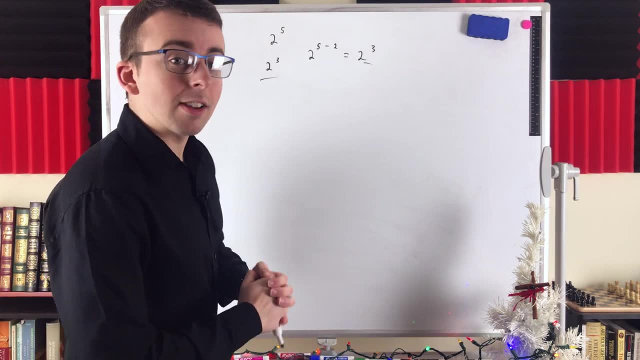 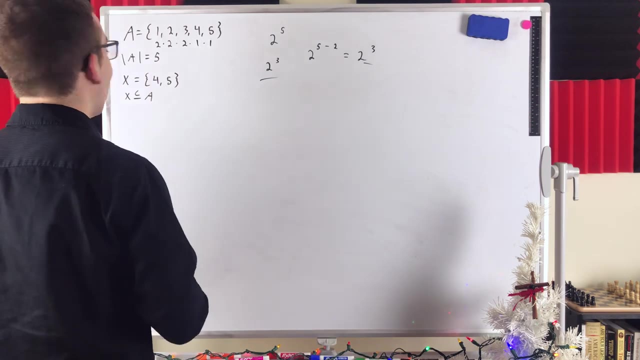 five, because we're guaranteeing they won't be included. so just keep in mind that that that's an equivalent problem in terms of the solution, but we'll continue talking about the problem in terms of including these elements. just keep that in mind. Okay, let's head on to the general. the general: 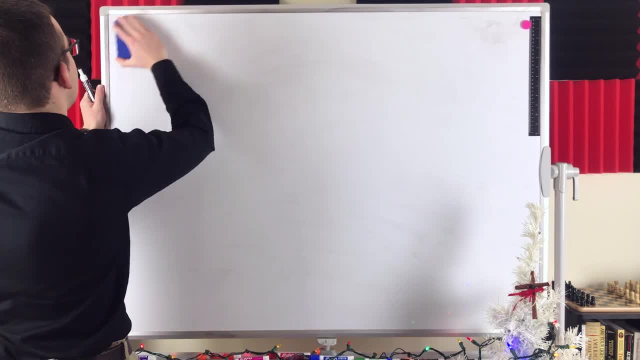 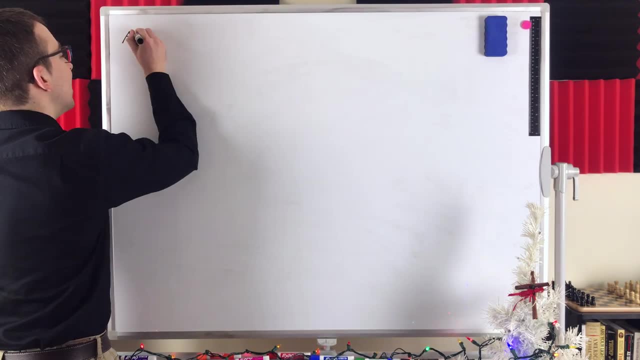 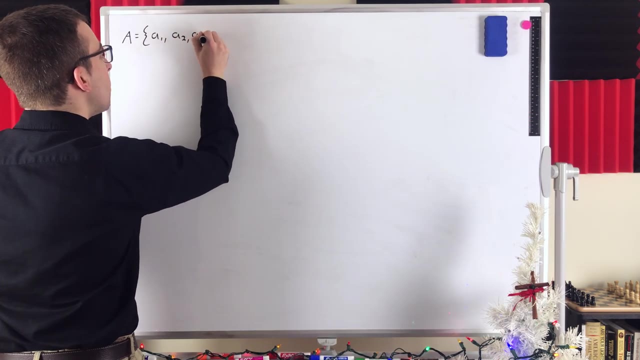 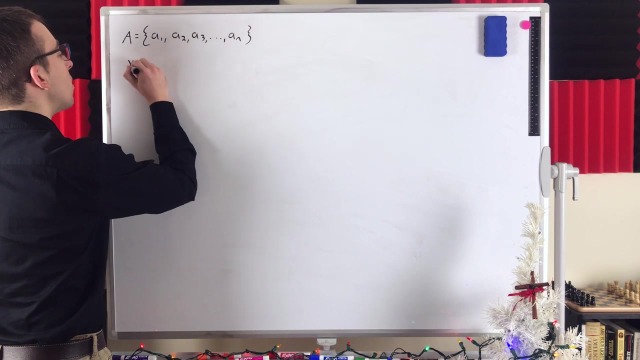 solution and then we'll call it a day. hopefully we can get through the rest of this without the train squealing again. All right, so let's say we've got a set A that contains n elements, so it's a finite set. say it contains the elements a1, a2, a3 and so on, some element a, n, then take an. 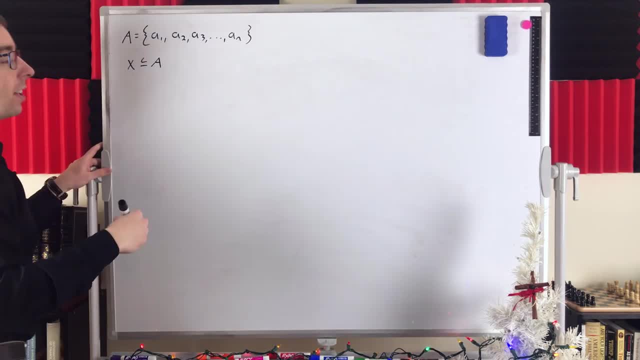 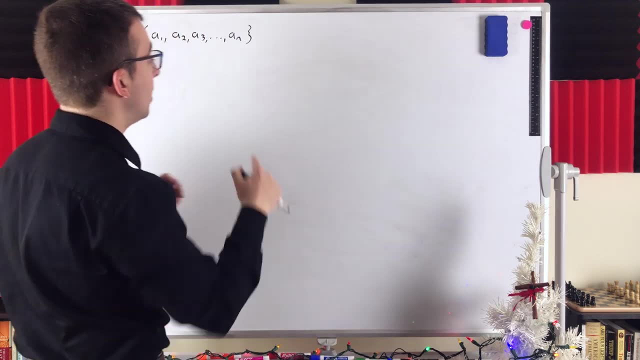 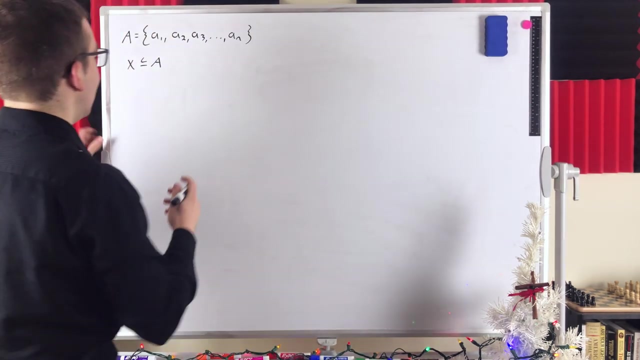 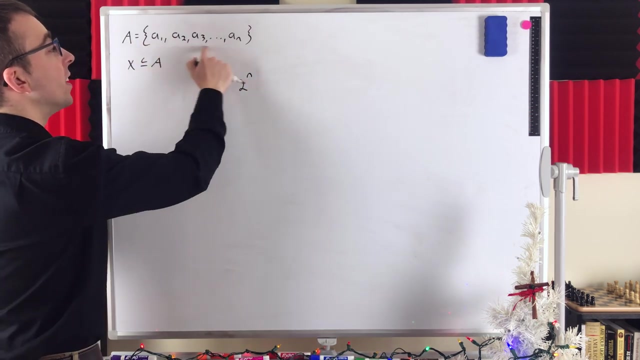 arbitrary subset of a called x. how many subsets of a? is x also a subset of? how many subsets of A contain all of the elements of X? The answer, as we just saw, and we can easily justify it in the general case, is 2 to the power of n, That's two choices for all n elements of A. 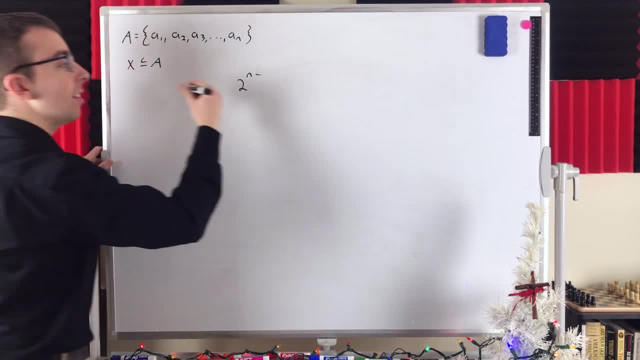 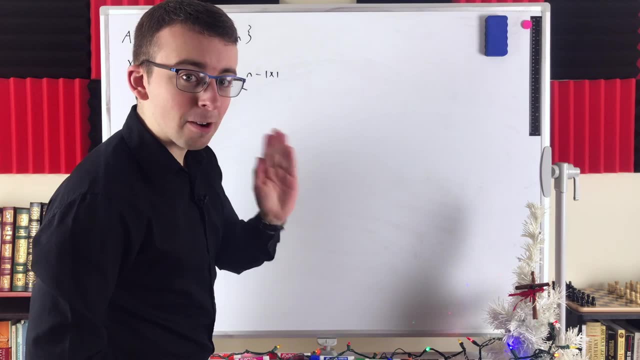 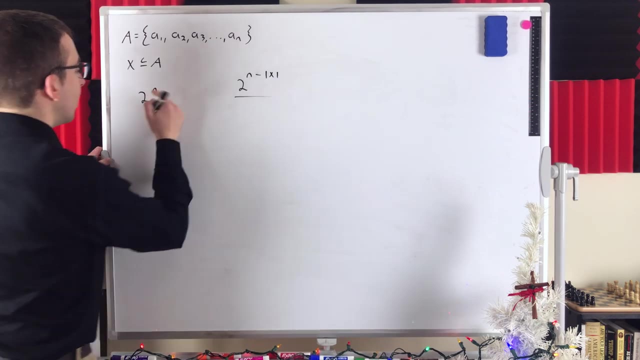 but then we have to subtract the number of elements in X, the cardinality of X, because we only have one choice for all of those elements that we're guaranteeing we will include. That's the answer. We could think of this as the total number of subsets 2 to the power of n two. 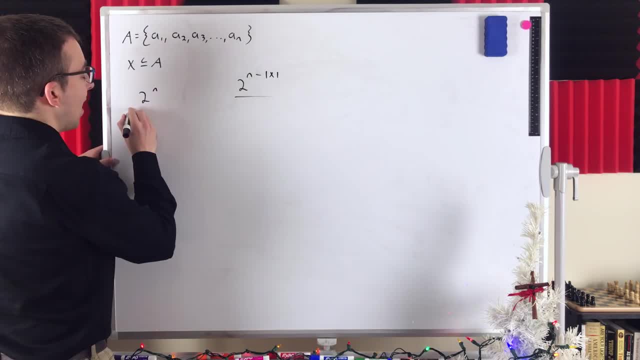 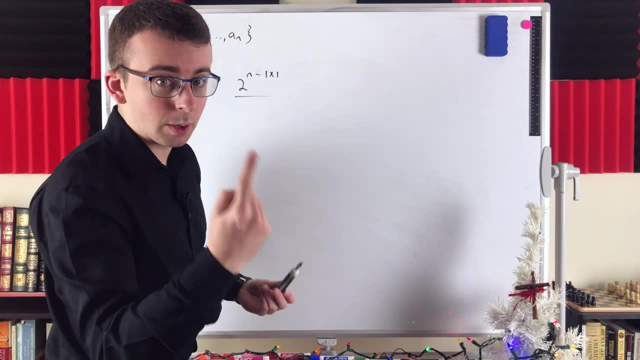 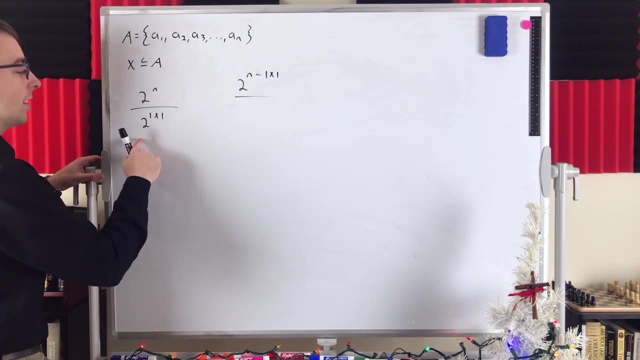 choices for all n elements. but then we have to divide out all of those factors of 2 for the number of elements that we don't have two choices for, We only have one choice for them. We would divide out 2 to the power of the cardinality of X, because that is the number of elements. 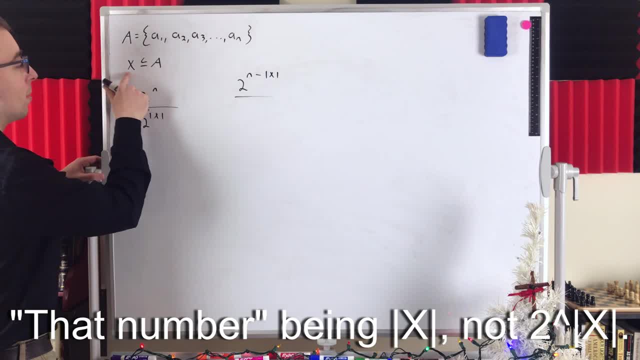 2 to the power of the cardinality of X. That's the number of elements that we only have two choices for. That's the number of elements that we only have two choices for, one choice for, because, again, we're guaranteeing we will include them, if you remember your exponent. 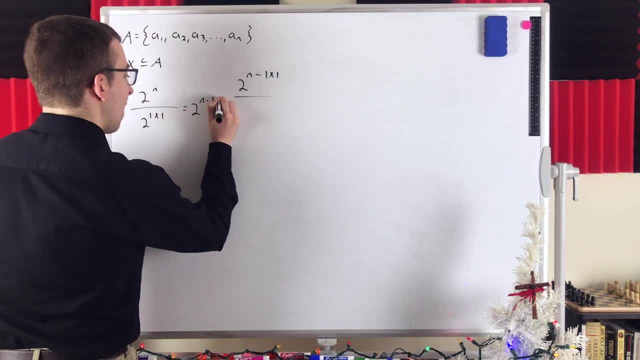 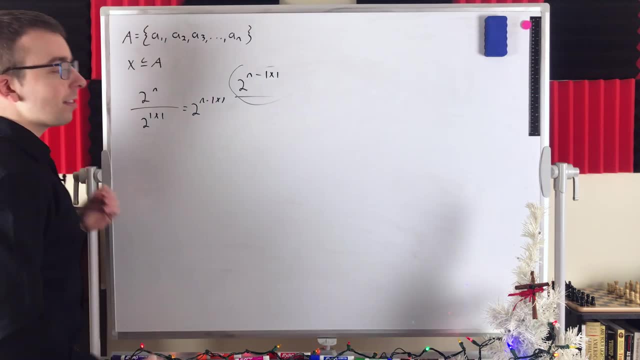 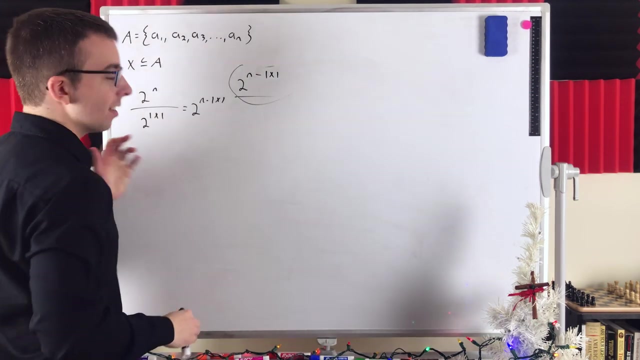 rules. of course, this is 2 to the power of M minus the cardinality of X. that's our answer. given a set with n elements and a subset of that set, X, with, of course, cardinality of X elements, the number of subsets of a containing all elements of X is 2 to the power of N minus the cardinality of X. 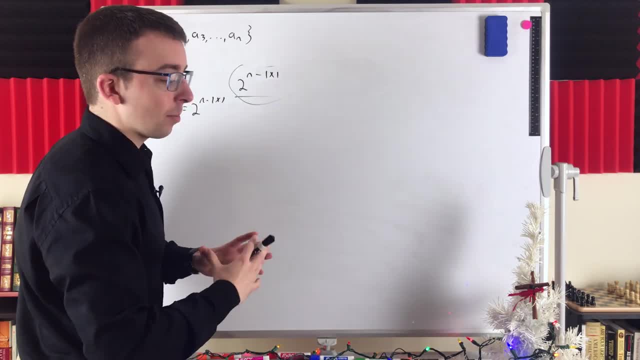 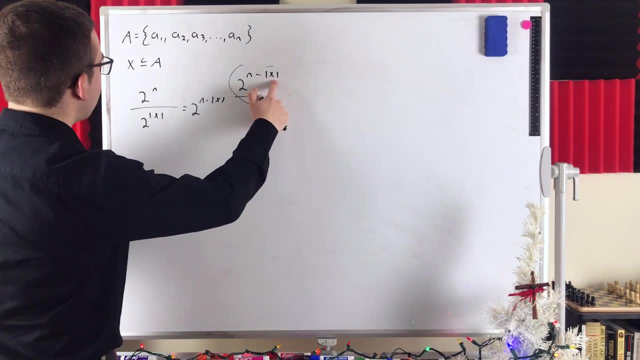 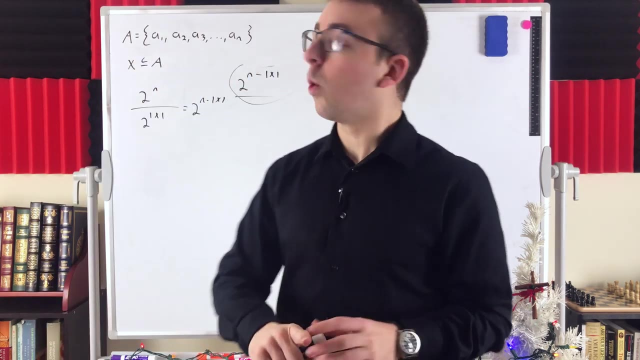 we can do a couple quick tests for some extreme cases. for example, suppose that X is equal to a, then the cardinality of X is equal to M. this becomes 2 to the power of 0, which is 1, which makes sense. there's only one subset of a containing all elements of a, which of. 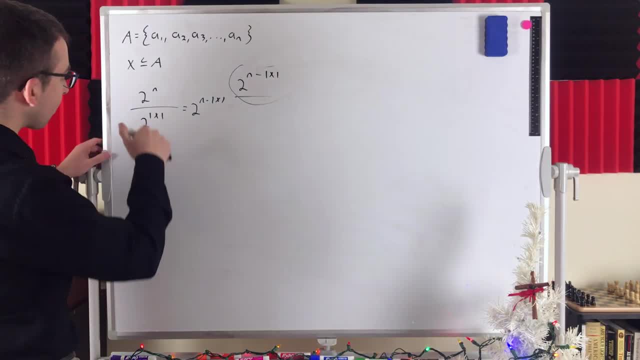 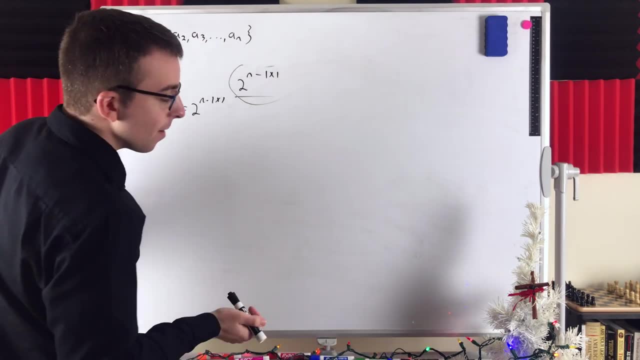 course, is the cardinality of X. if we want to think about that- and what we would do is we would- is a Another extreme case we might check is if x is the empty set, which is possible because the empty set is a subset of a, Then the cardinality of x is equal to zero. This is just left as 2 to. 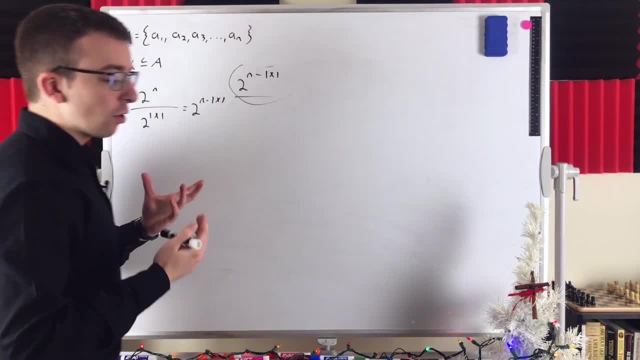 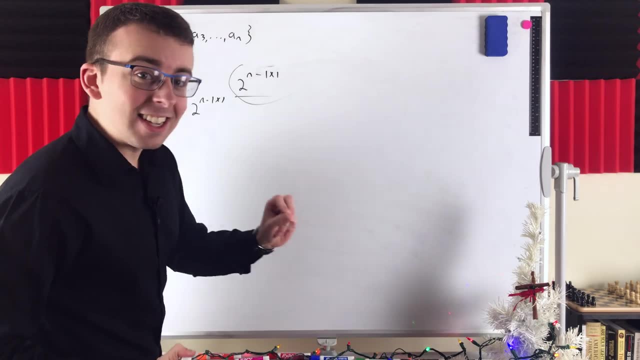 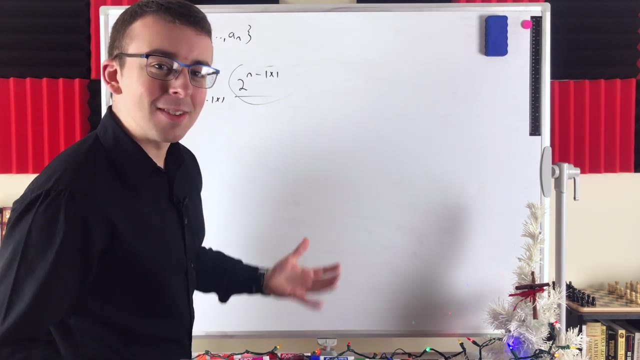 the power of n, And so that should make sense. 2 to the power of n is the answer, That's the total number of subsets of a that are guaranteed to contain the elements of the empty set. In other words, we're not guaranteeing anything because the empty set has no elements. So of course, 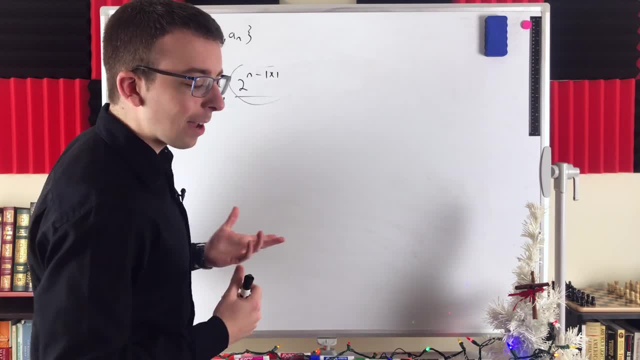 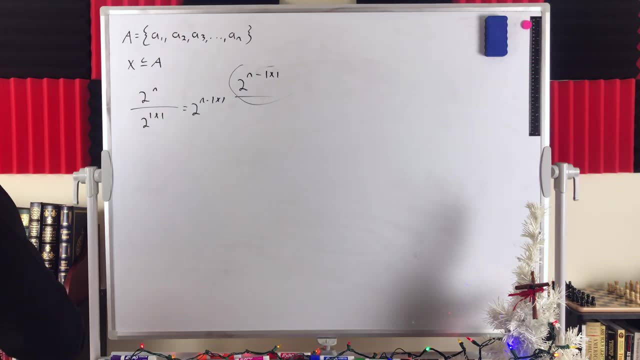 guaranteeing that your subsets must include the elements of the empty set doesn't reduce the number of subsets at all, because the empty set has no elements And I guess we can leave it there. I suppose I'll leave you with an example problem. Let's say we've got a set S. 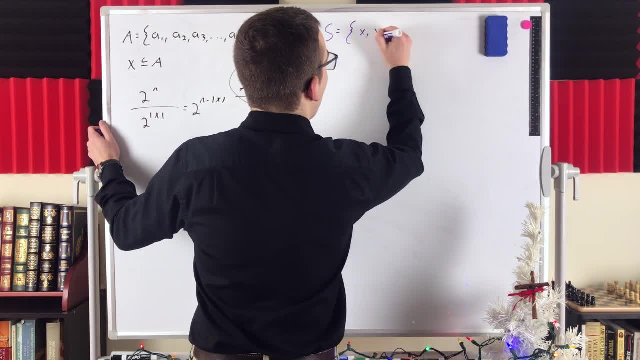 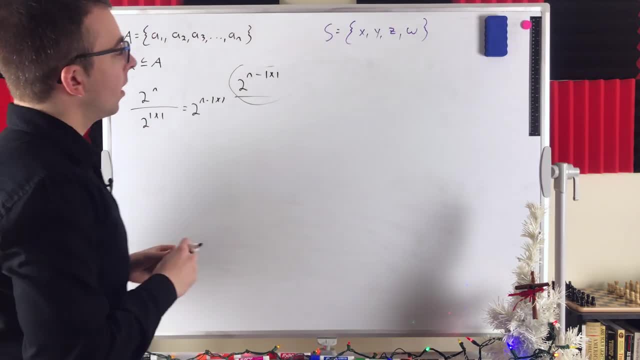 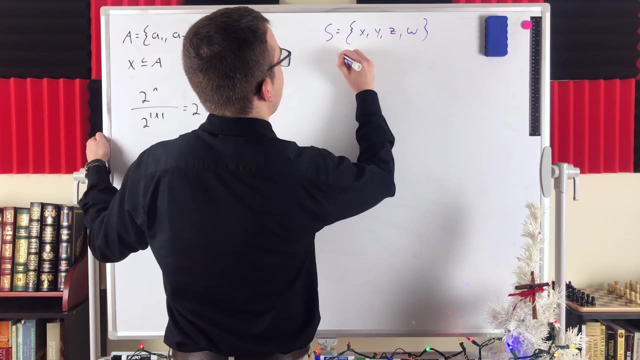 containing the elements x, y, z, and let's throw in a w, x, y, z and a w. Riddle me this: how many subsets of s are there containing the elements of this set? We'll call this set r. 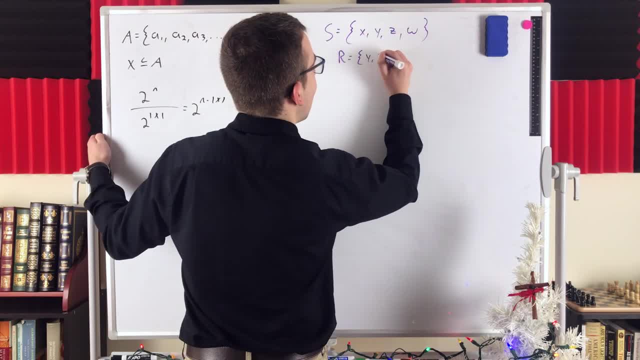 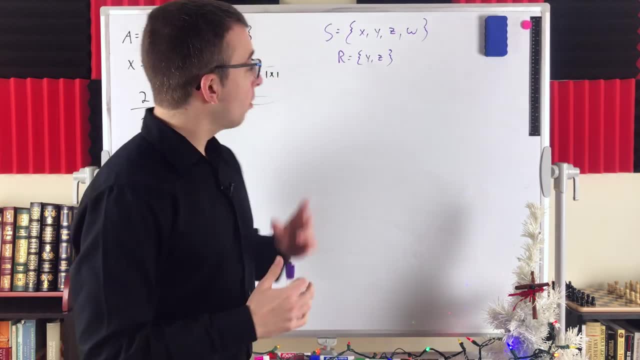 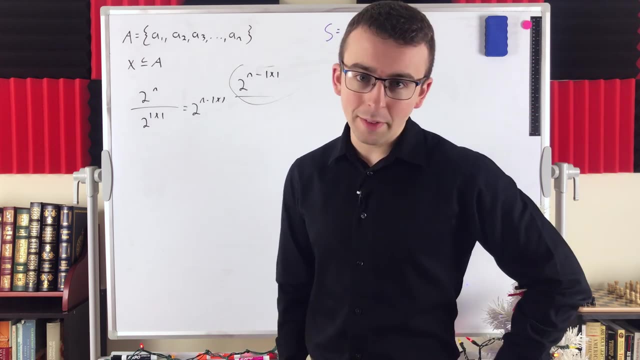 How many subsets of s are there containing the elements y and z? Let me know in the comments. I'll leave the solution in the description. So I hope this video helped you understand how to solve this pretty fun little set counting problem. Let me know in the comments if you have any. 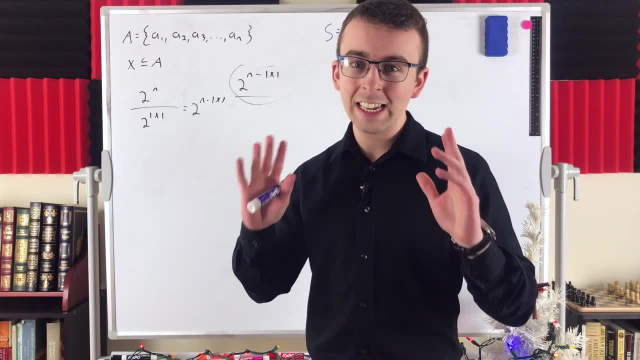 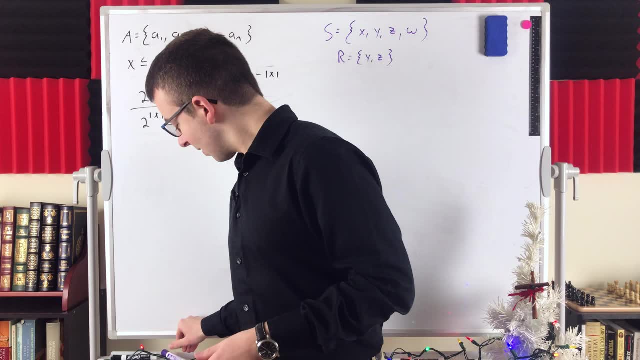 questions, need anything clarified or have any other video requests? Thank you very much for watching. I'll see you next time and be sure to subscribe for the swankiest math lessons on the internet. And a big thanks to Valo who, upon my request, kindly gave me permission to use his